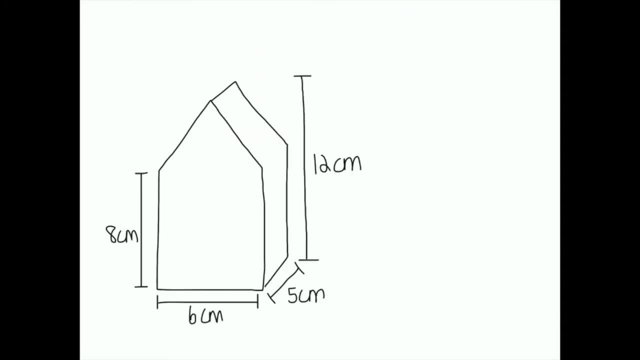 This is the shape that I'll be using. I can see that the entire shape is 12 centimeters high and it has a base with measurements of six centimeters and five centimeters. I can see here. just looking at the shape, it looks like it can be divided into two shapes. 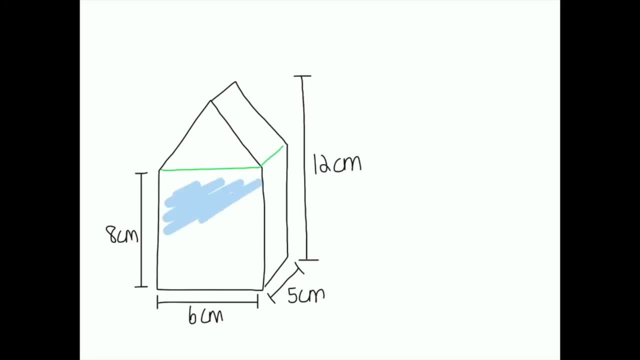 I can see a rectangular prism which I'll shade here in blue, and I can also see a triangular prism up the top which is shaded in purple. If I draw this out, I have my rectangular prism and I have my triangular prism. I can see that my rectangular prism has measurements of five centimeters by six. 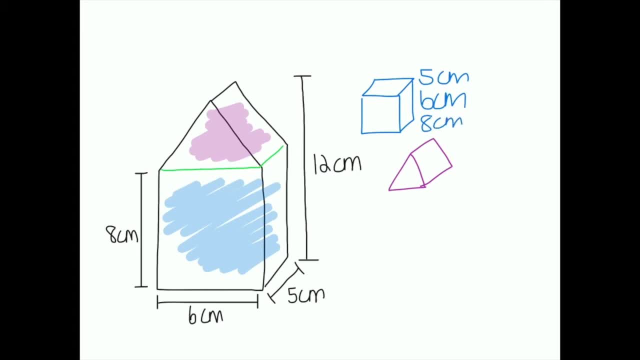 centimeters and it is eight centimeters tall. For my triangular prism I can see that its base is six centimeters and its perpendicular height, which is here, is four centimeters, because I have 12 centimeters for the entire shape and eight centimeters for the height of that rectangular. 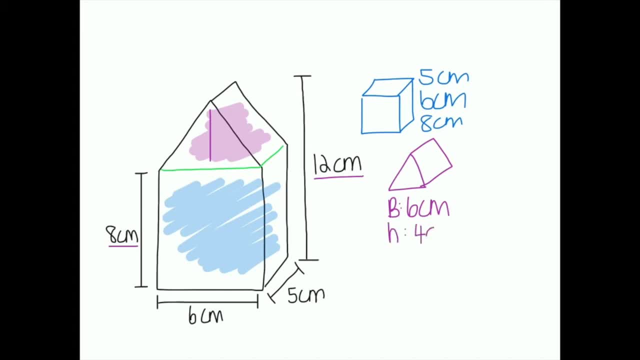 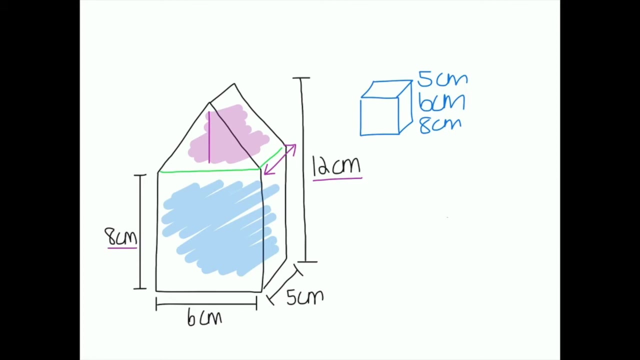 prism. So I'm going to go. height is four centimeters and I know that going this way, which I'm going to call that height with a capital H, is five centimeters. The first calculation that I'm going to make is the volume of the rectangular prism. The formula to calculate the volume of a. 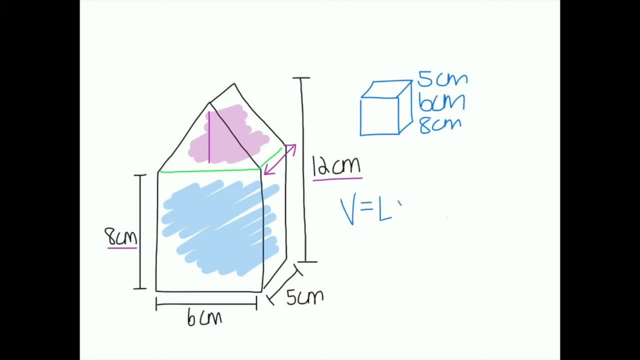 rectangular prism is: volume equals length times width, times height. So I'm going to say that my length is five centimeters, my width is six centimeters and my height is eight centimeters. Five times six is thirty times eight, Three times eight is twenty-four and times that by ten gives: 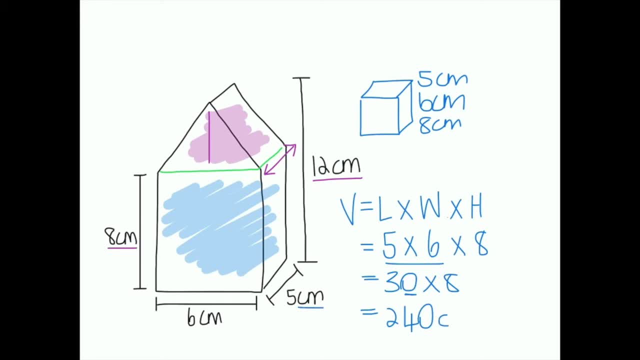 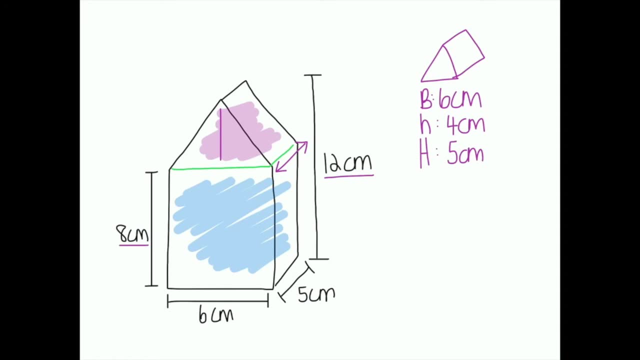 me 240.. I'm dealing with centimeters and I'm dealing with volume, so that measurement is cubed. The second calculation that I'll be working out is the volume of the triangular prism. The formula to calculate the volume of a triangular prism is: V, equals base times, height divided by two. 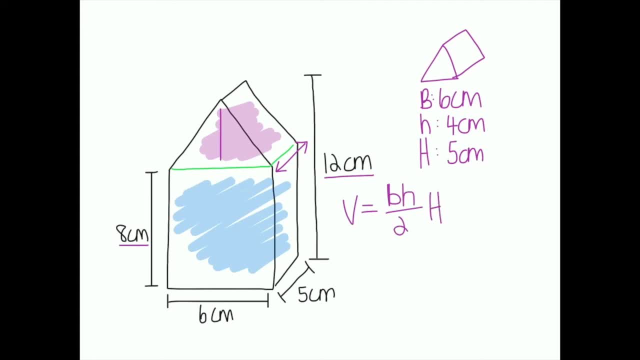 times the height of the prism. So I know that my base length is six centimeters and that the perpendicular height is four centimeters. So I'm going to be timesing that, then dividing it by two, but I also have to be sure that I'm multiplying that section.